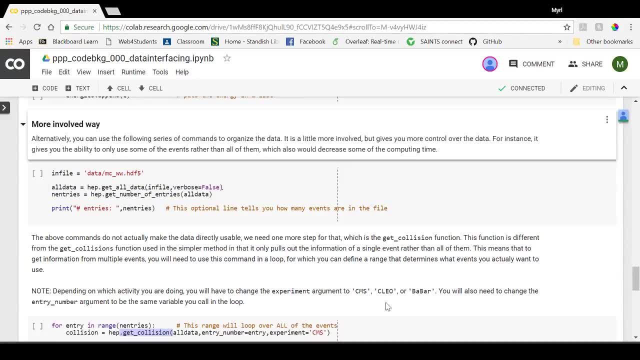 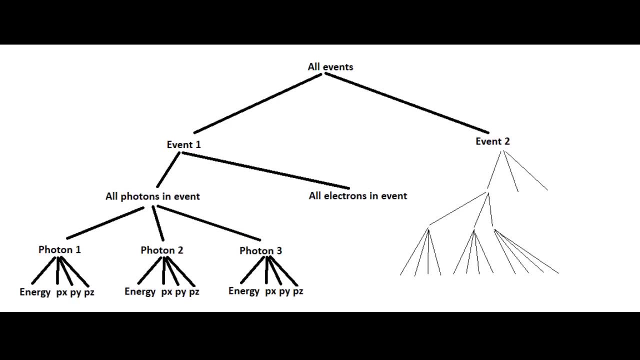 Whichever of these functions you use, they both organize data into lists the same way. Here is a quick visual representation of how the data is structured. Here at the top is your whole data file, which is a list of every collision event that occurred- Each event. 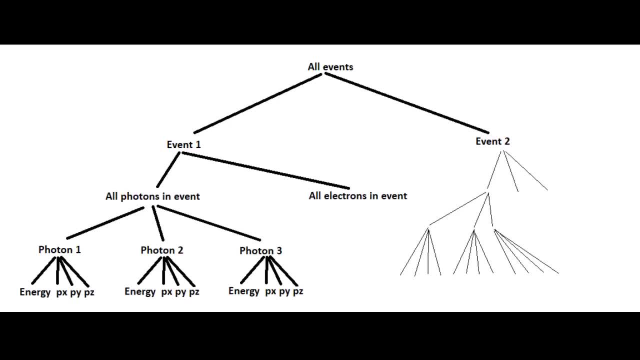 is also a list. For instance, if you looked at the first event in the file, you would see that it is a list of every type of particle involved in that collision: Electrons, photons, muons, etc. Each of these particle. 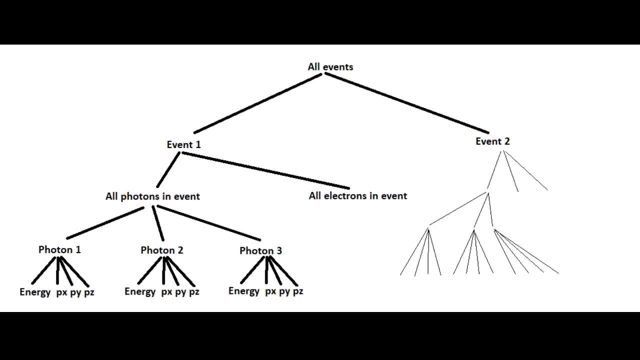 types is another list of all the particles of that type which were in the collision. For instance, there may be five photons in the whole collision. And finally, each individual particle is another list of all the characteristics of that particle. As an example, this individual photon will have information about its energy and x, y. 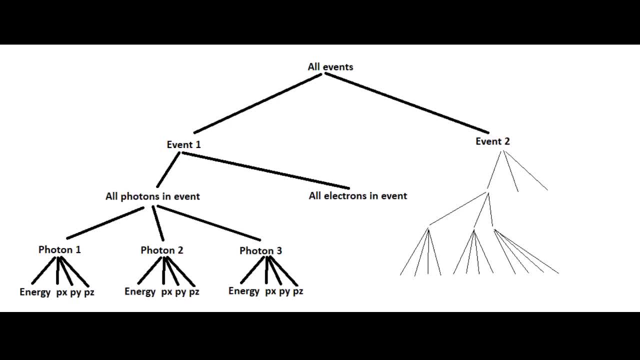 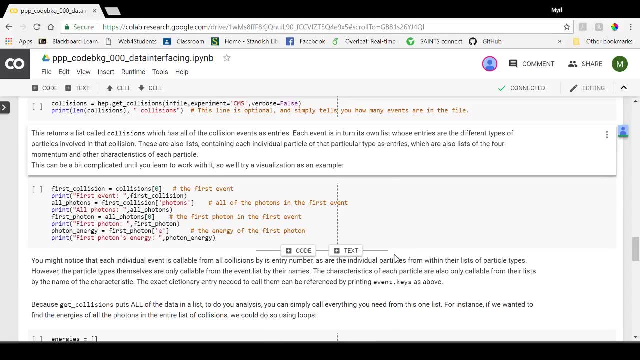 and z momentum. Other particles may have more information, like charge and b-tag. The entries from these lists are callable either with their index numbers or according to their dictionary keys. The events are called by their index number, so the first event would be collisions. The types of particles are called by the name of that. 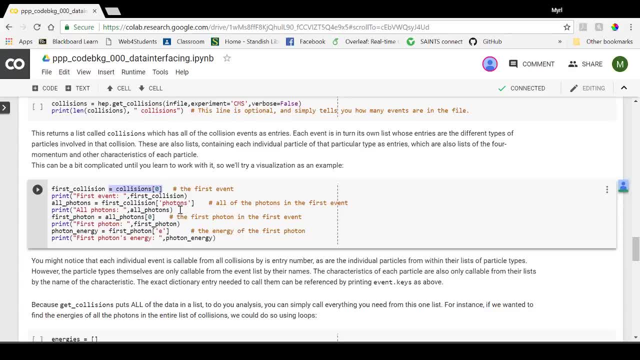 particle type. so the list of all photons in that event would be called by first event: photons. Each of the individual photons are then called by their index number, so the first photon in that list would be photons. Finally, the characteristics of that particle. 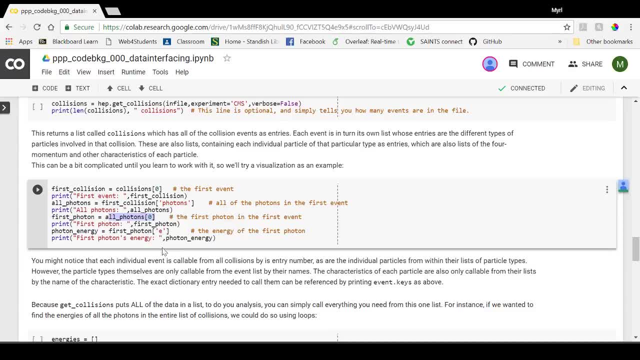